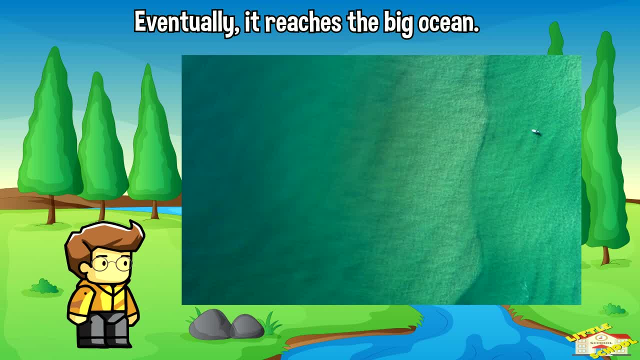 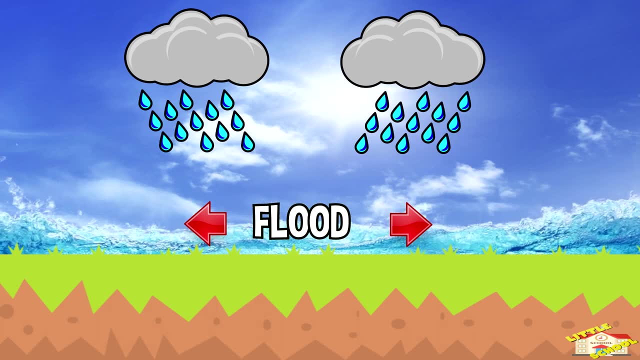 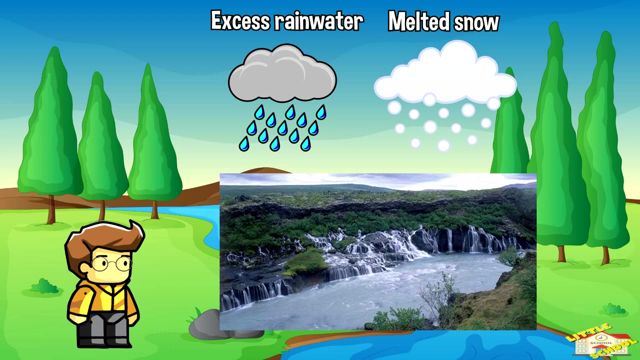 the big ocean. When it rains a lot and there's too much water racing around, it can cause problems Like flooding. Surface runoff is the movement of water over the land surface when excess rainwater, melted snow or other sources of water do not infiltrate into the ground or evaporate. This 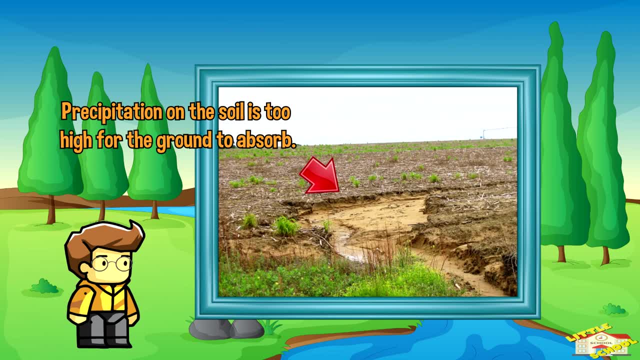 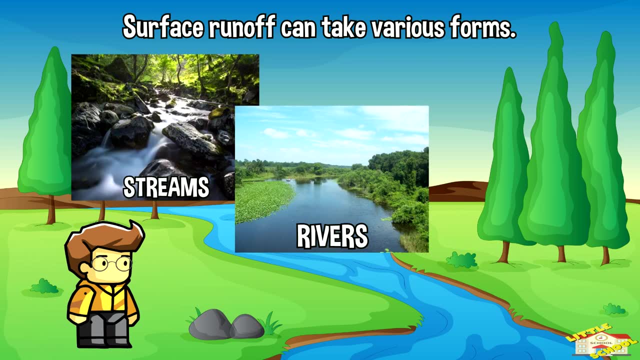 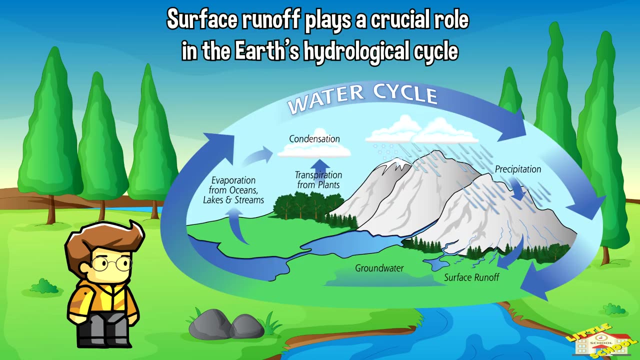 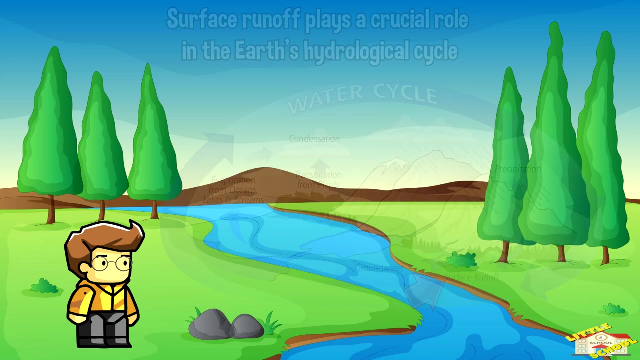 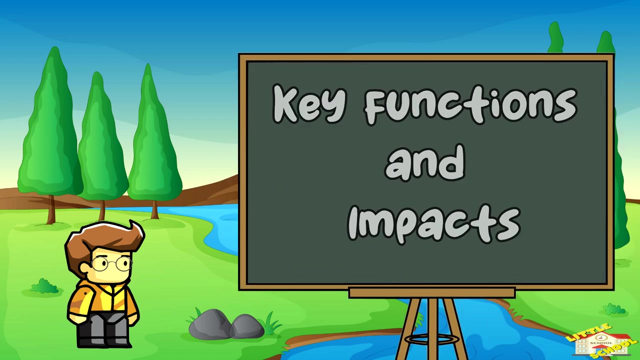 runoff typically occurs when the rate of precipitation on the soil is too high for the ground to absorb. Surface runoff can take various forms, such as flowing in streams, rivers and creeks. Surface runoff plays a crucial role in the Earth's hydrological cycle. Both can have natural and human-induced consequences. Some of its key: 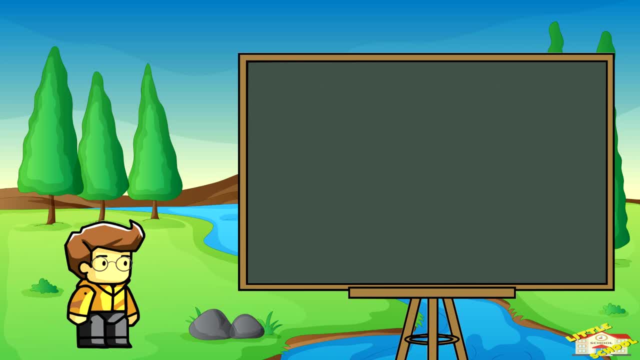 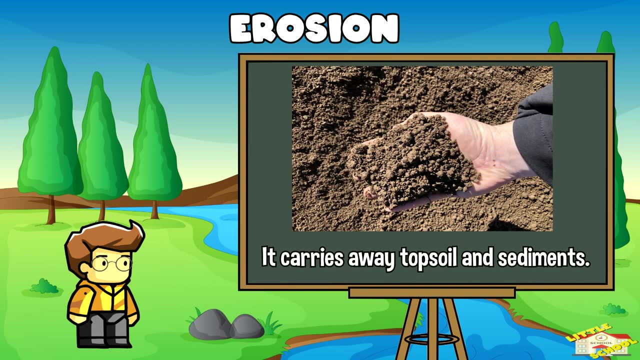 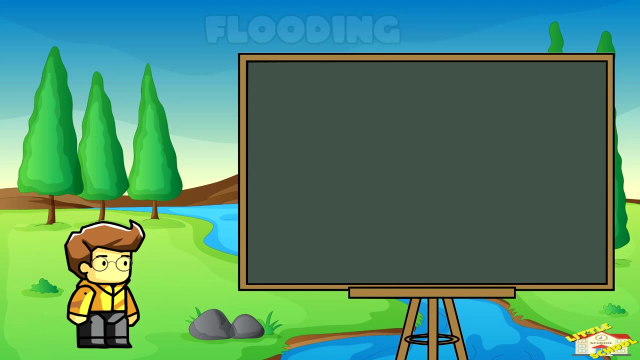 functions and impacts include: erosion: Surface runoff can lead to soil erosion. It carries away topsoil and sediments, which can be detrimental to agriculture. Flooding: When surface runoff is excessive, it can result in flooding in low-lying areas. 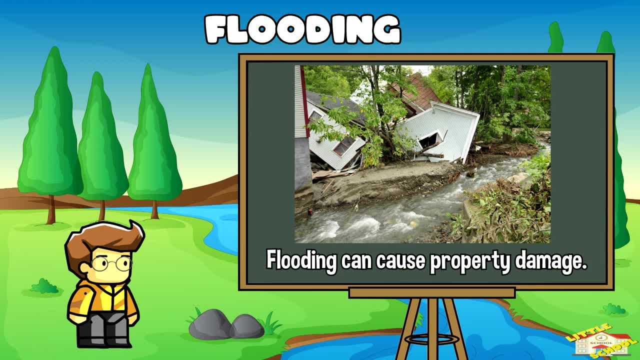 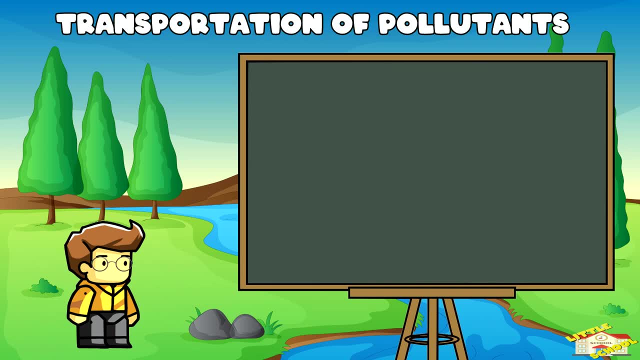 Flooding can cause property damage and pose a threat to human safety. Transportation of pollutants: Runoff can pick up and transport pollutants such as fertilizers, pesticides and other pollutants. Surface runoff can also cause soil erosion. Surface runoff can also cause soil erosion. Surface runoff can also cause soil erosion. Surface runoff can create. 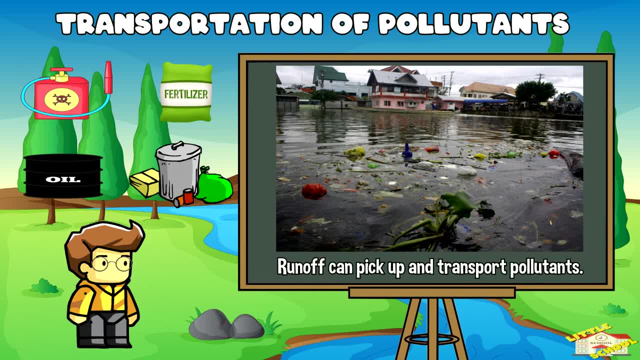 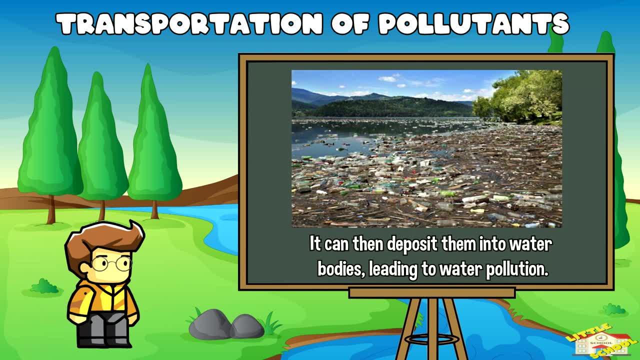 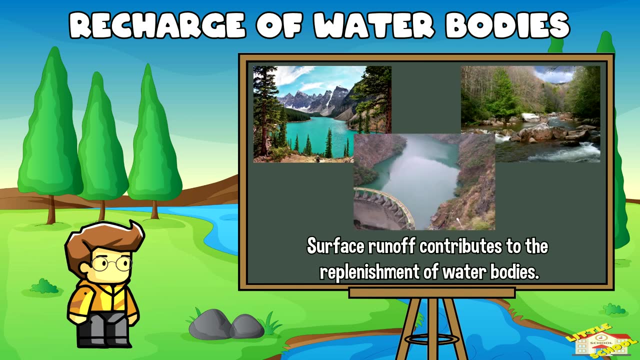 water and sediment desertification. Surface runoff can catch water, ash and other pollutants, such as pesticides, oil and litter from roads and urban areas. It can then deposit them into water bodies, leading to water pollution. Recharge of water bodies. Surface runoff contributes to the replenishment of lakes. 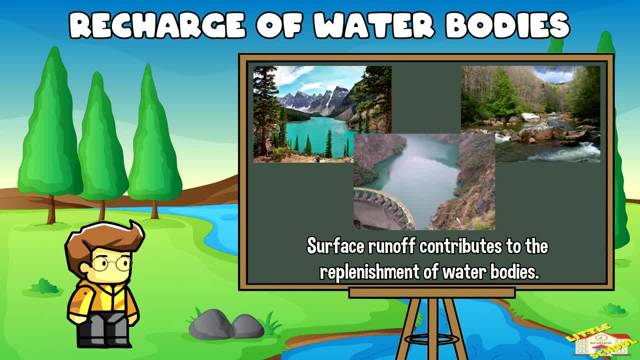 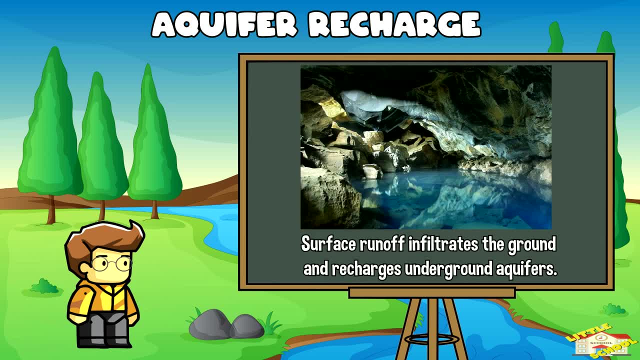 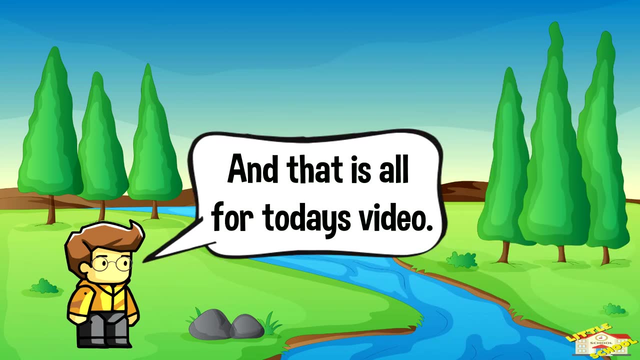 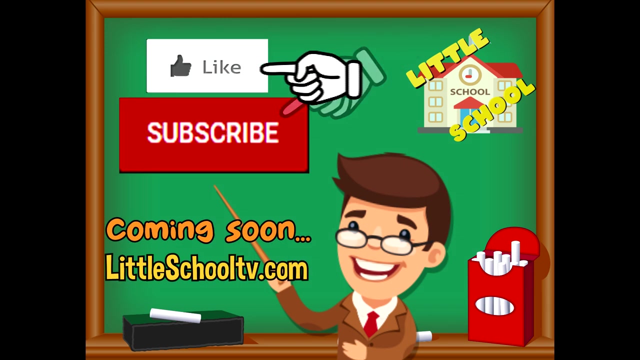 rivers and reservoirs Aquifer recharge. In some cases, surface runoff infiltrates the and recharges underground aquifers. and that is all for today's video. I hope you enjoyed learning about surface runoff today. take care now, bye. bye. if you enjoyed a video and want to see more videos from us, please click the.